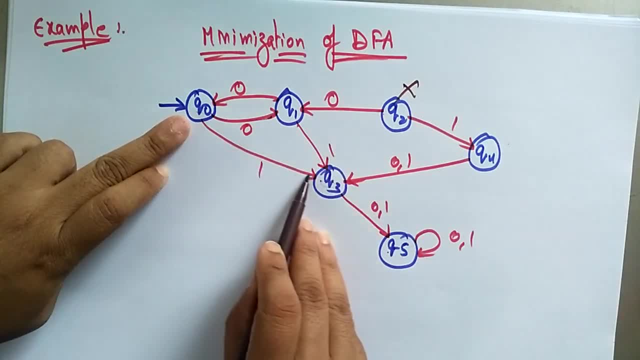 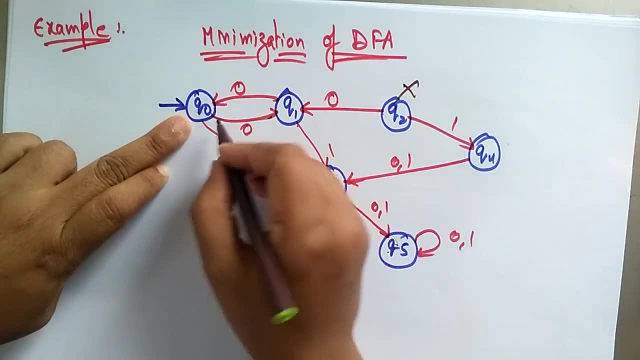 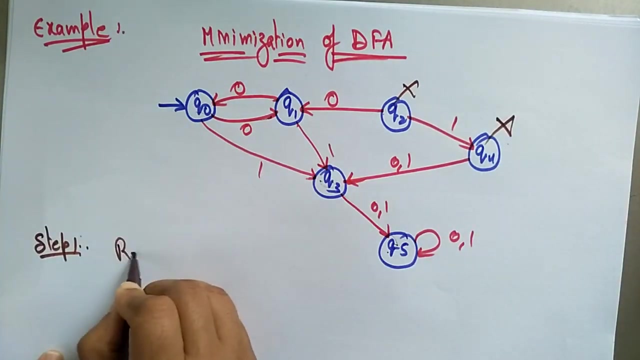 no, there is no possible. And come here From this way: Q3 and Q5. I am going to Q5, but I am not going to Q4. So from initial state I am not able to reach the Q4 states. So just remove. remove Q2 and Q4 in. 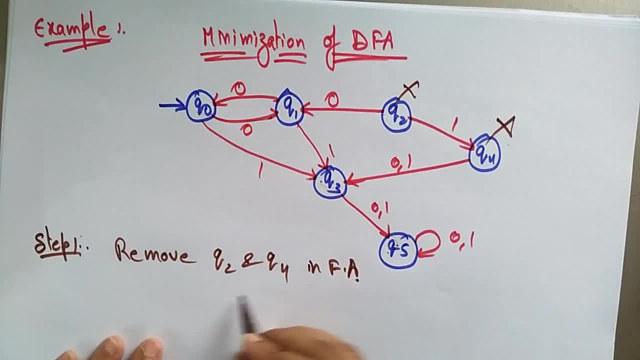 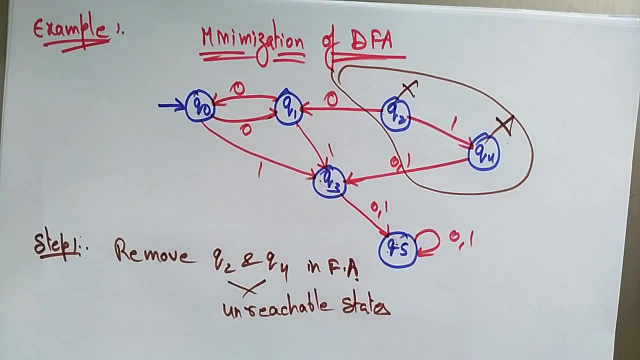 finite automata. Okay, because these are unreachable state. unreachable states. Okay. so now these, these two are are removing from the state, So I will get only the four states: Q0, Q1, Q2, sorry, Q0, Q1, Q3 and Q5.. So what is the second step? I need to draw the. 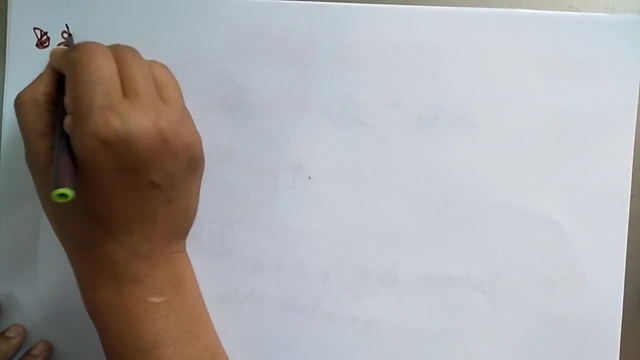 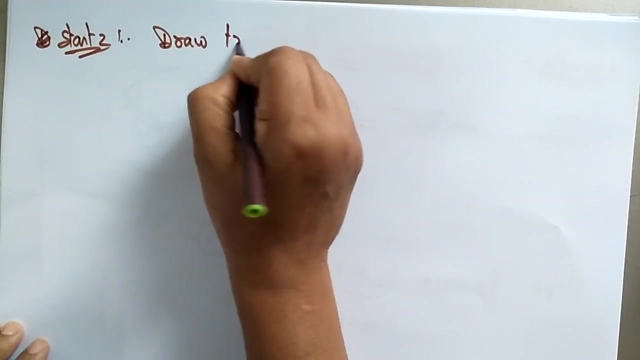 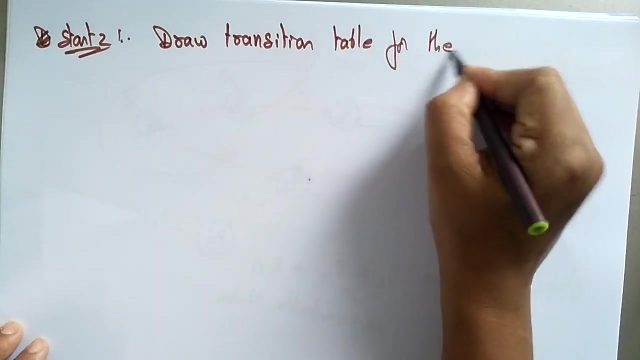 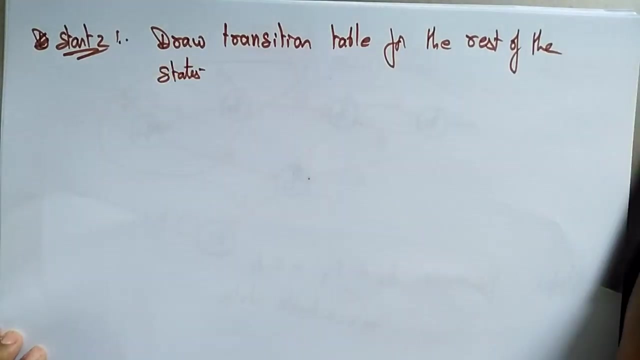 transition table. So after drawing the transition table, don't don't need to check the diagram. Okay, so draw. After removing the unreachable states, I need to draw the transition table For the rest of the states. for the rest of the rest of the states. So states 0, 1.. Okay, 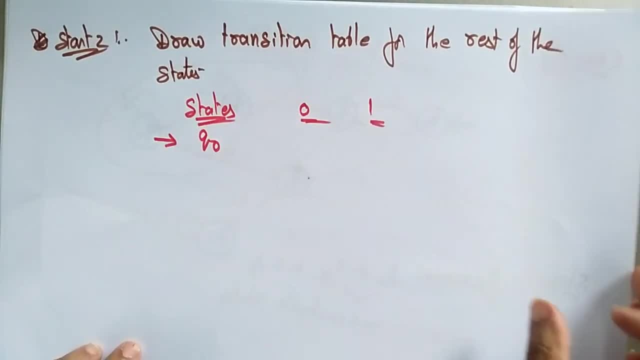 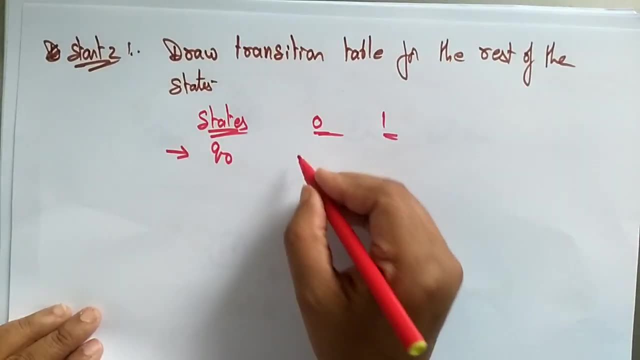 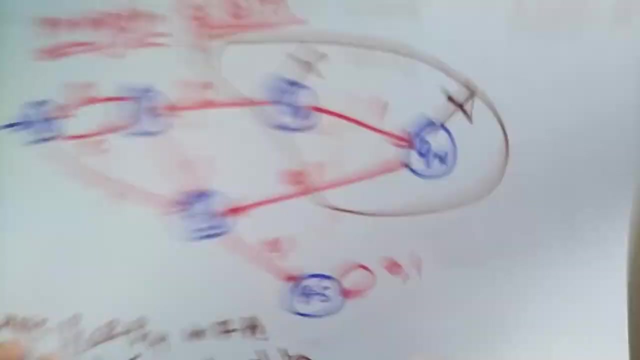 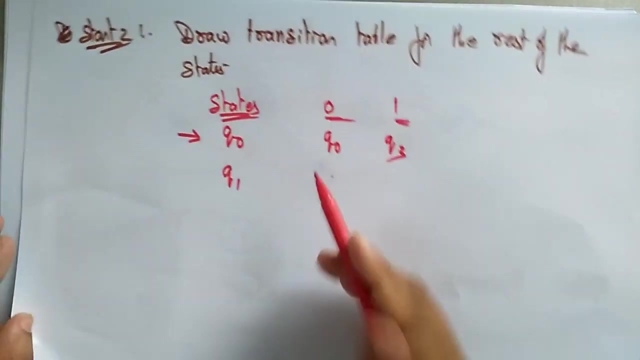 So Q0 is the initial state. I know that. Now let me check: Q0 on 0 going to Q1 and Q0 on 1 going to Q3.. So this is Q0, Q3.. state is q1. so q1 on 0 goes to q0 and q1 on 1 goes to q3. q0, q3. so in the same way I am writing. 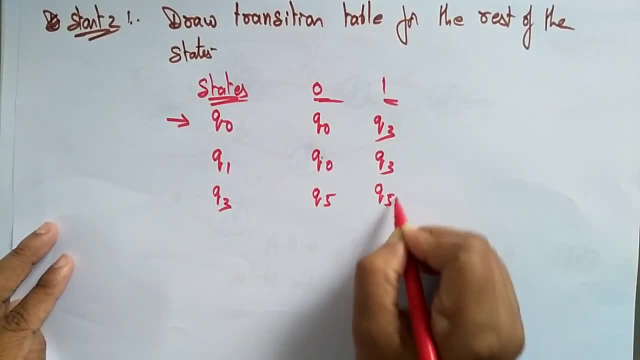 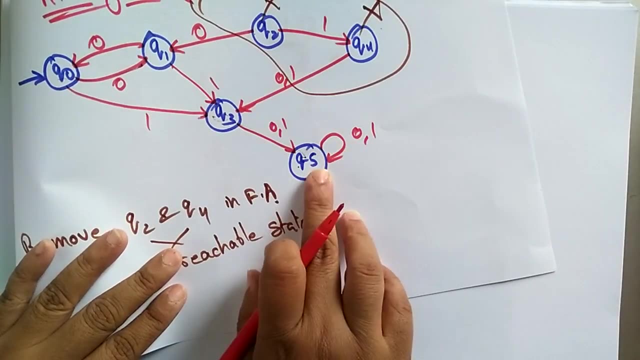 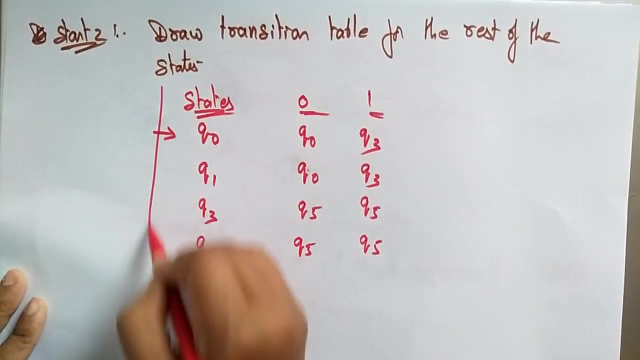 for the remaining states also: q5, q5, and in the same way, q5 is going to q5 on. so q5 on 0 going to q5, q5 on 1 going to q5 itself. okay, so now I constructed the transition table. so now, 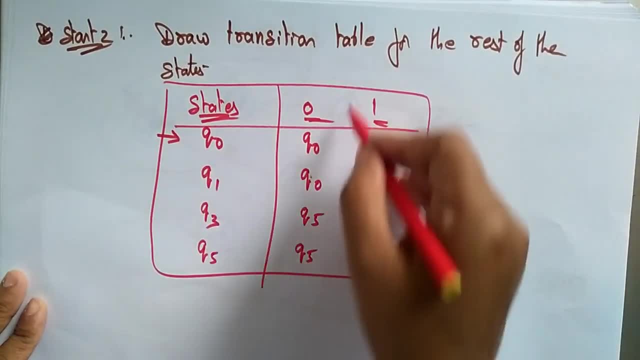 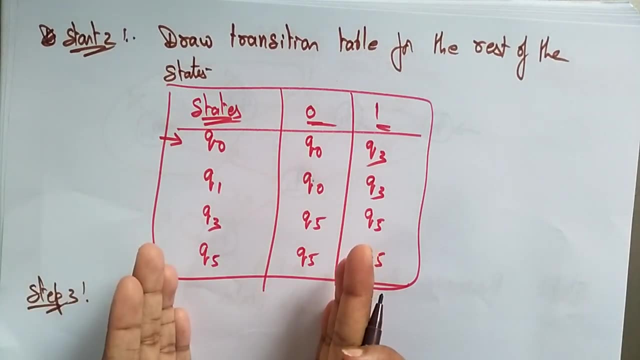 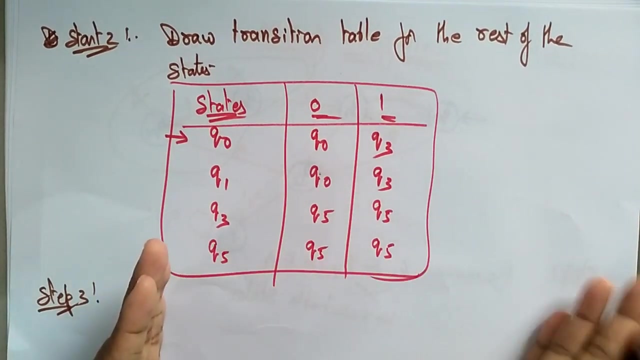 what is that? the next step three, step three. what is the step three? according to our algorithm, divide the table into two tables. now, divide the table rows of a transition table into two sets. one is the t1 and the t2, so one transition is of starts with. 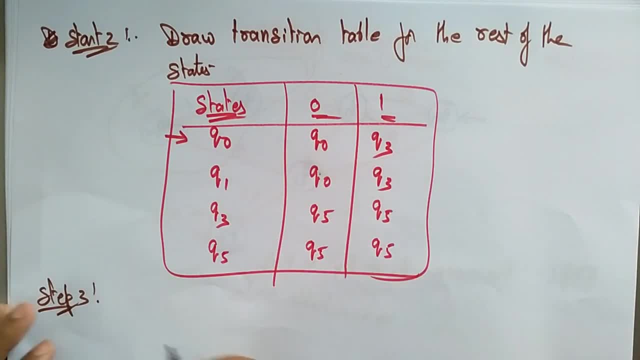 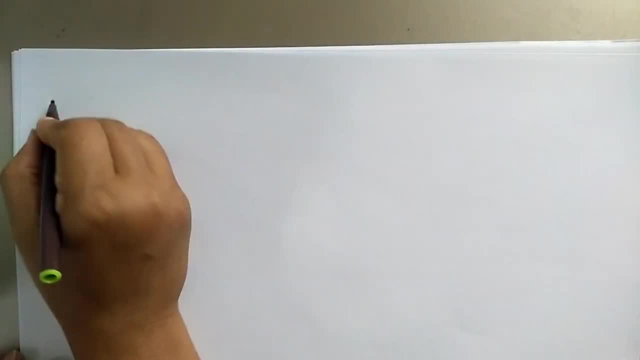 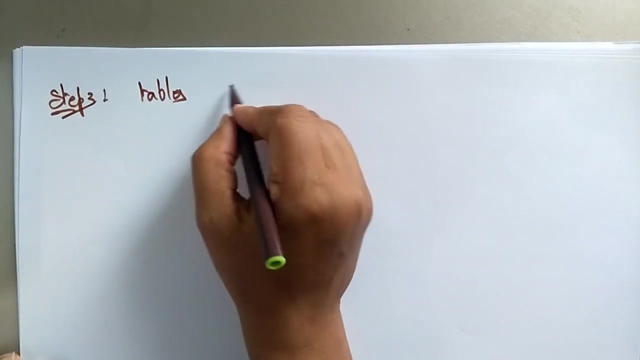 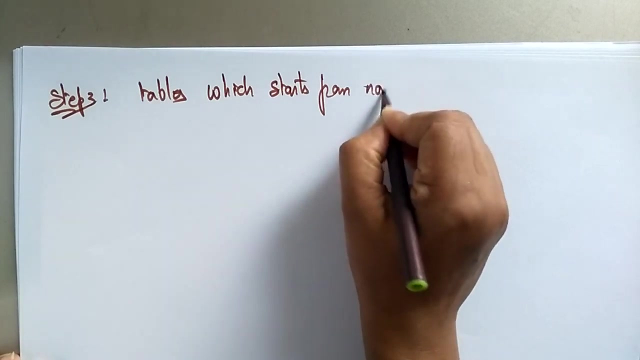 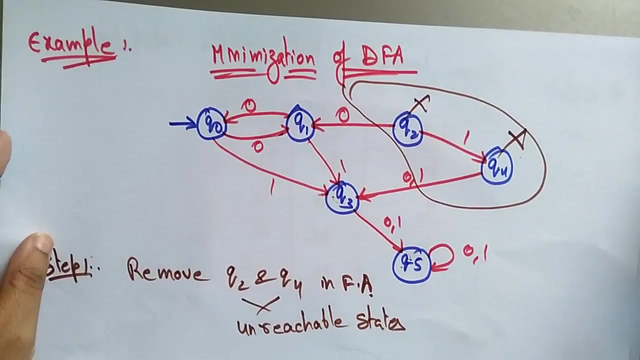 table which starts from non-final states table. let me take the fresh page, step three, table which from which starts from non-final states, non-final states. so what are the non-final states? so here the final states are. sorry, i didn't write the final states, only the initial state. i have written q naught is initial state and here the final states are q3. 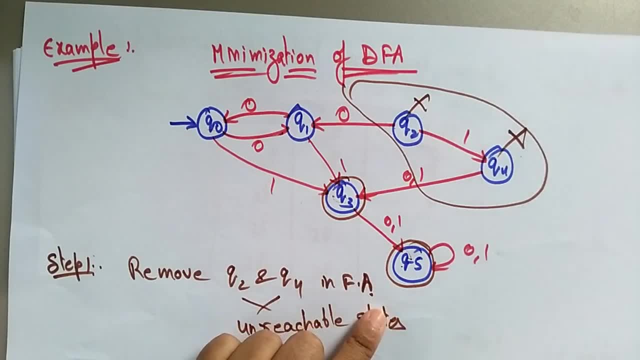 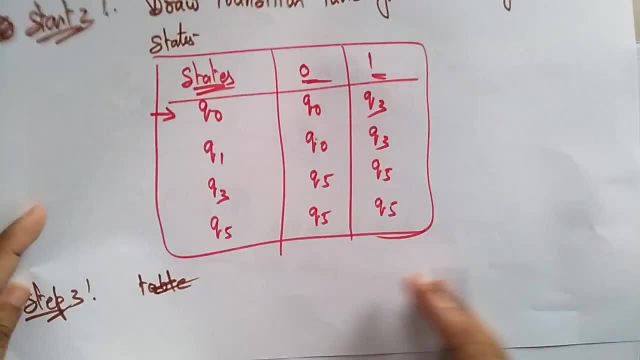 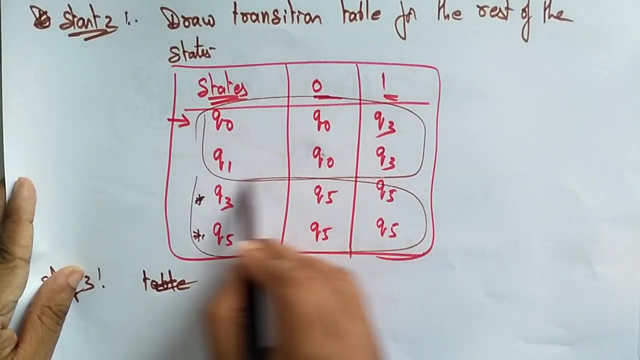 and q5. two of these two are the final states. so what are the final states? the final states are q3 and non-final states. what are the non-final states? these two are the final states. so these two comes under one table and these two comes under the another table. so i am splitting these. 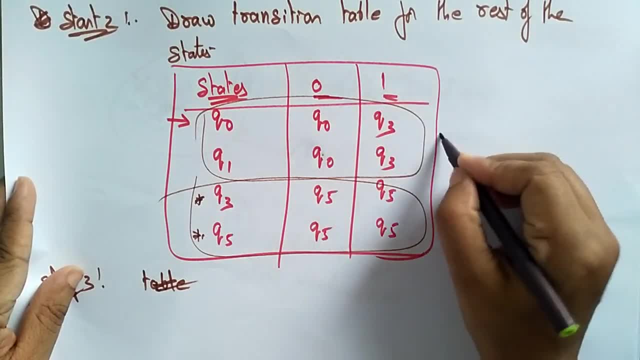 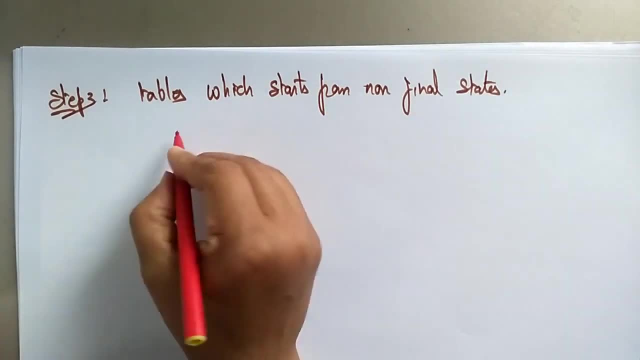 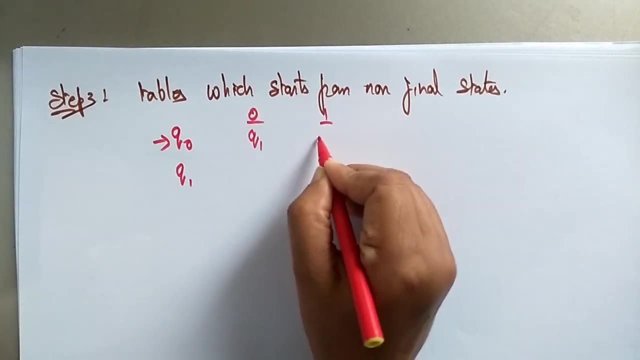 two: these are the non-final states and these are the final states. so i am taking t1 and the t2 tables which start from non-final states, or q, naught and q1, so on 0 and 1 it goes to q1 and q3, q naught and q3, so another table. 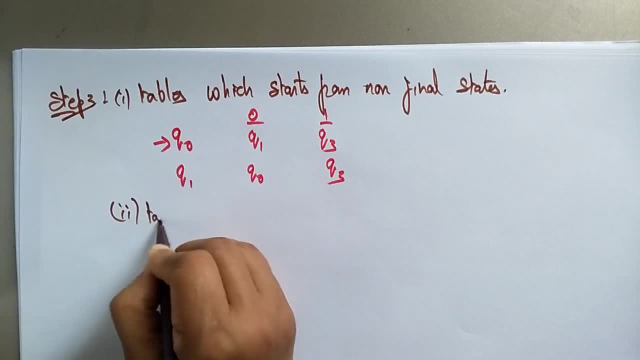 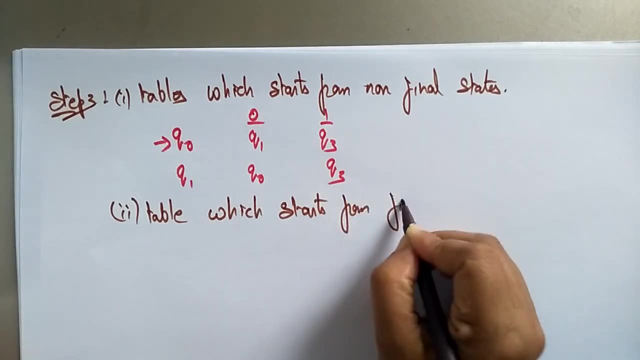 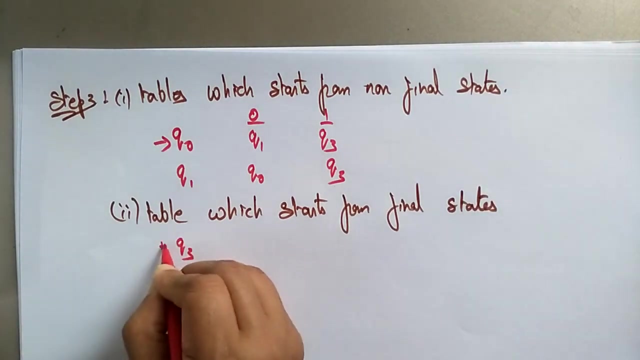 tables. table which starts from: from final state. so that is q3 and q5. these are final states: 0, 1 on 0, it is going to q5. here also q5, q5, q5. so now coming to the step 4. so what is the step 4? so i had taken the dfa. i removed the. 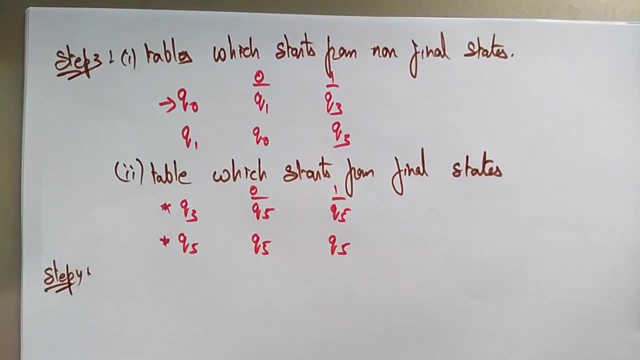 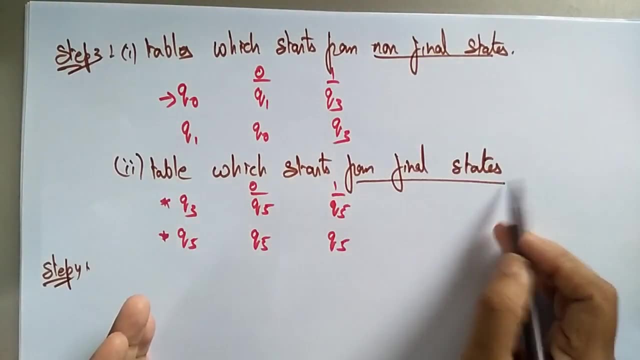 unreachable states. after that, i had drawn the transition table and i had taken the unreachable table, so i after that i split the table into two tables: t1 and t2. one contains non-final states, another contains final states. okay, so now i need to check whether they are having the similar rows. 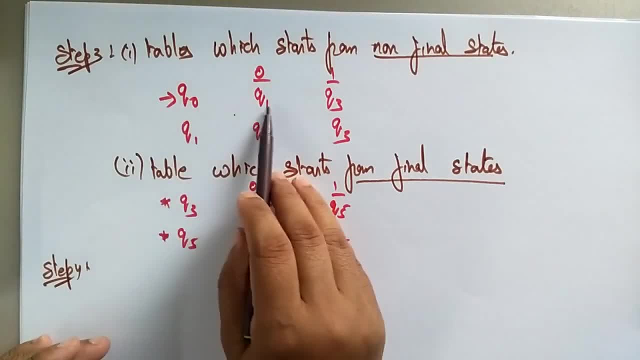 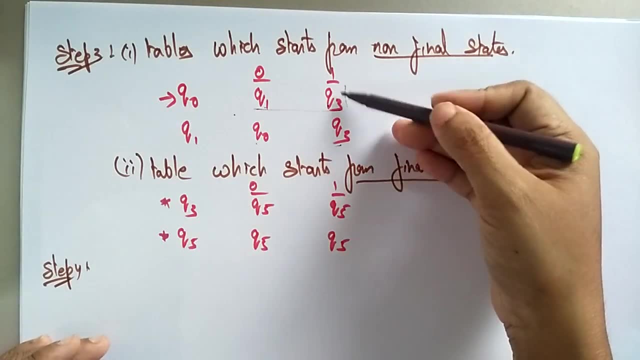 or not? so in this first table you are getting the similar rows q1, q3s, not similar. q naught, q3, not similar. these two tables are not similar. these two rows are not similar because here these two are same, but these two are not same. okay, you can see that these two rows are not same, but these two are. 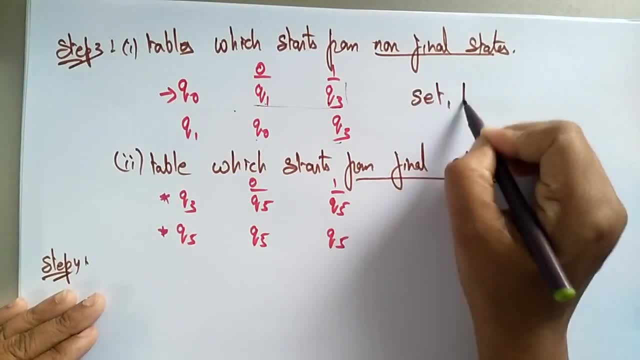 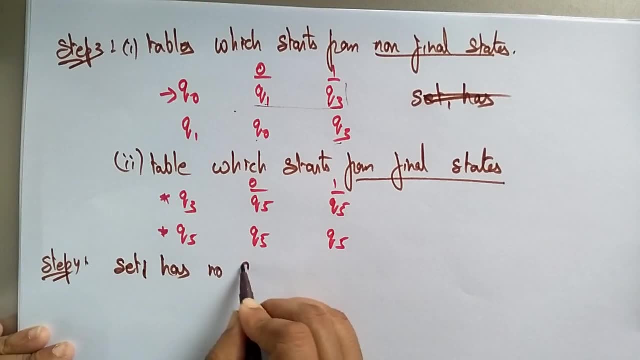 same, but these two are not same. but these two are not same, but these two are not same. so you can see, you can see, uh, set one has, set one has. let me write here in step four, step one: uh set one has no similar rows. okay, no similar rows, so they will be same. 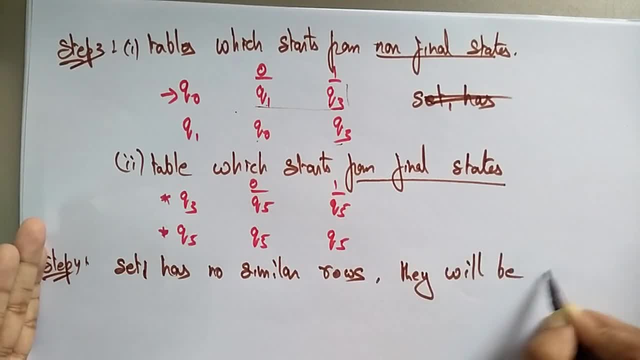 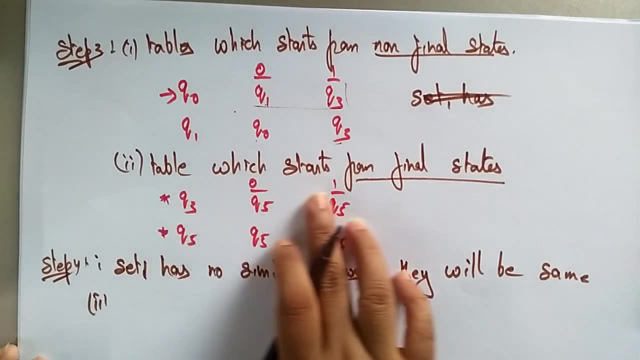 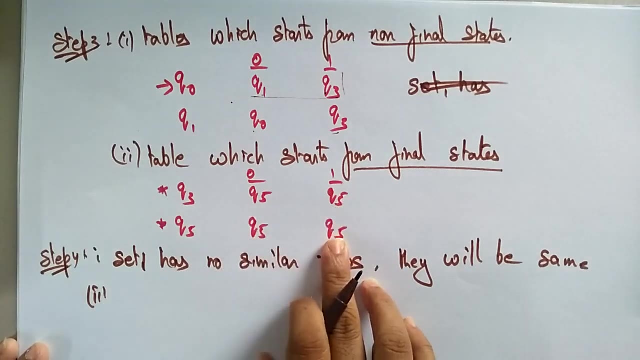 they will be same, so don't change anything in the this table. now coming to this table. so here this table. uh, this table has two rows having the same fields: q5, q5, q5, q5. so in the set two, the row one and the row two are similar, since q3, q5 transits, uh, to the same state: zero and one. 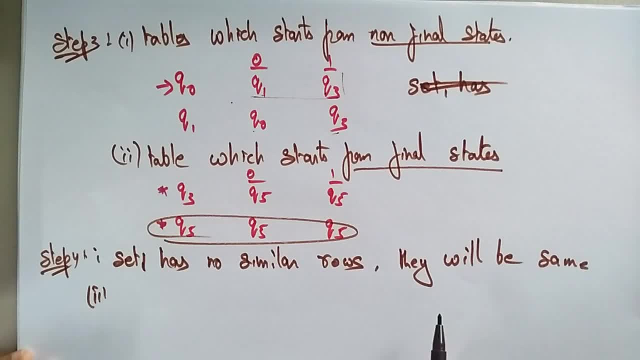 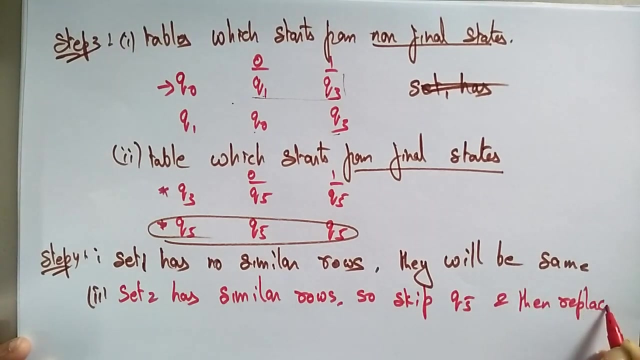 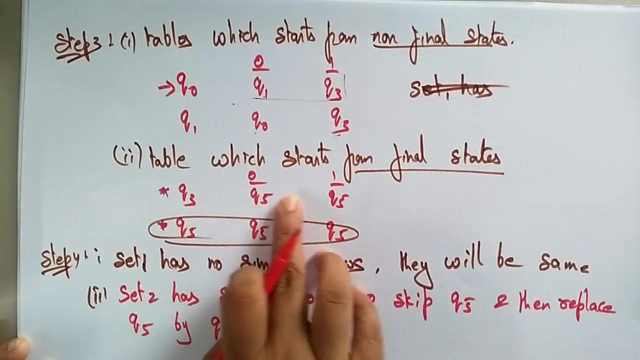 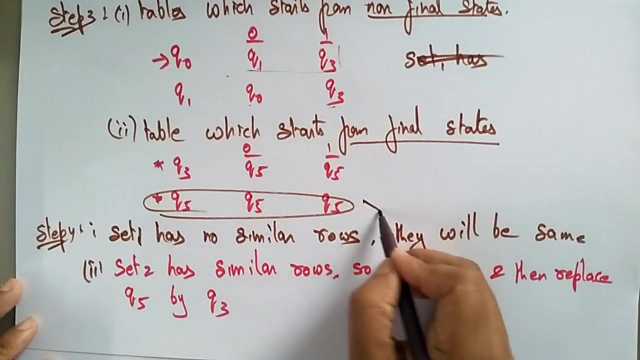 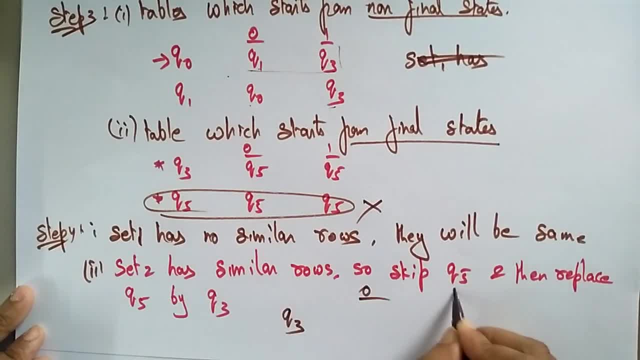 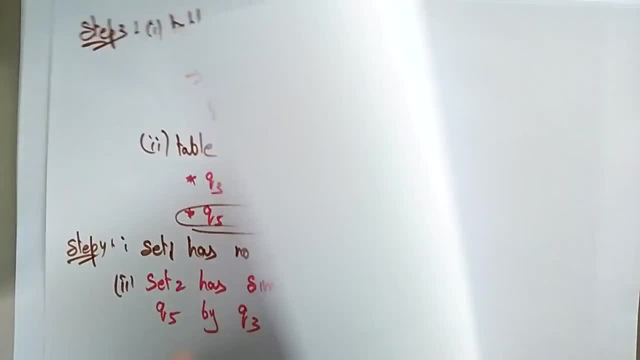 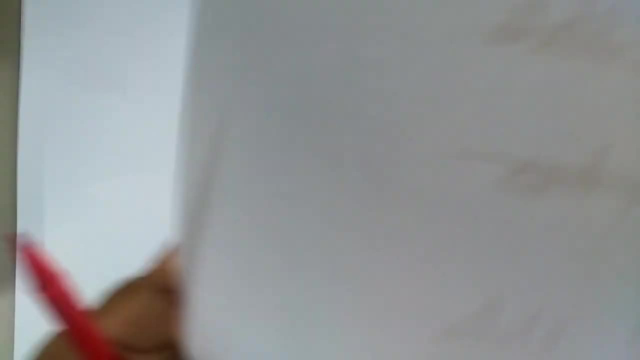 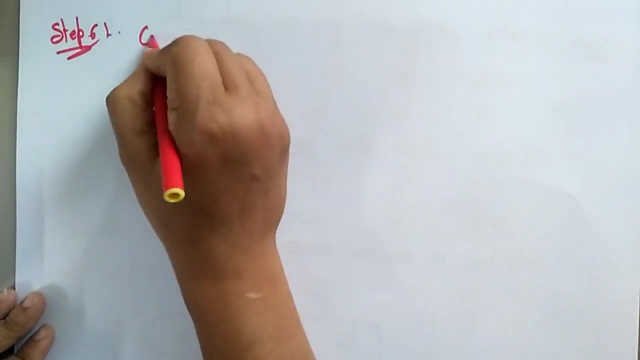 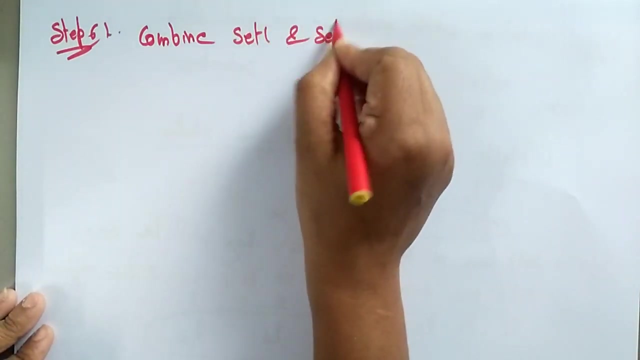 you will get Q3.. In the place of Q5, I have to write Q3, Q3.. Okay, Now combine the two rows. So this is my new table and this is another table. Now combine the table in the step 6.. Step 6. Combine set 1 and set 2.. After combining the set 1 and set 2, you will get. 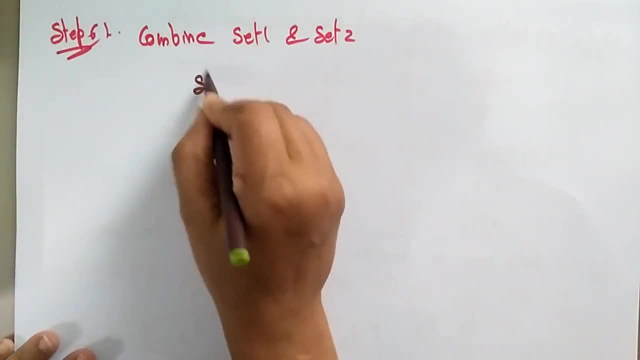 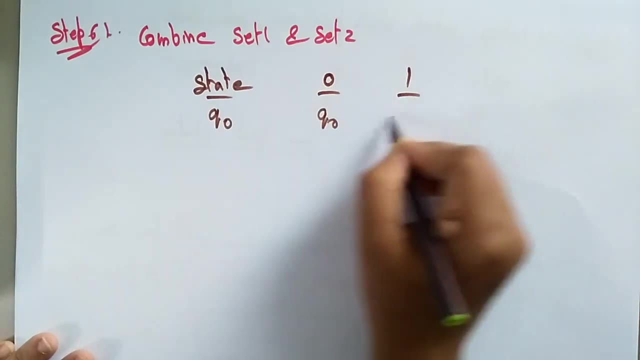 the new transition table. So what is the new transition table? with the state 0, 1.. So what is the state? The first table contains Q0.. I didn't change the first table because it is a new table. So I didn't change the first table because it is a new table. So